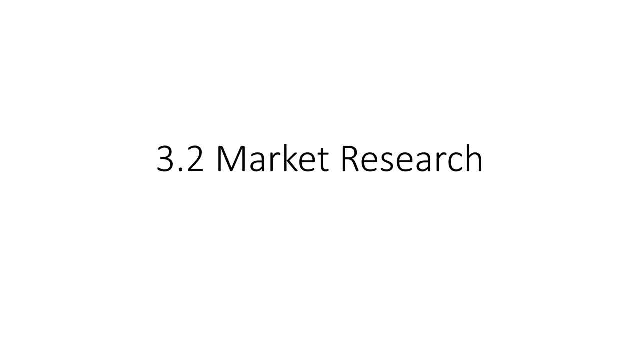 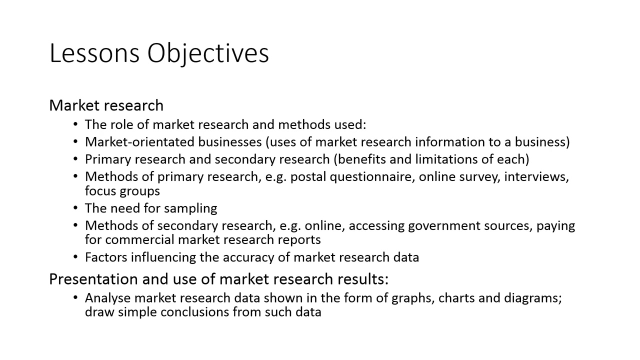 Hello everybody, welcome to Sense Business YouTube channel. Today we'll cover 3.2, market research. Please join me and I'll make sure you get the highest possible grades in your IJCC business exam. So today's lesson's objectives are market research. so the role of market research. We'll talk about market orientated businesses and we'll talk about product orientated businesses. We will also talk about primary and secondary market research. 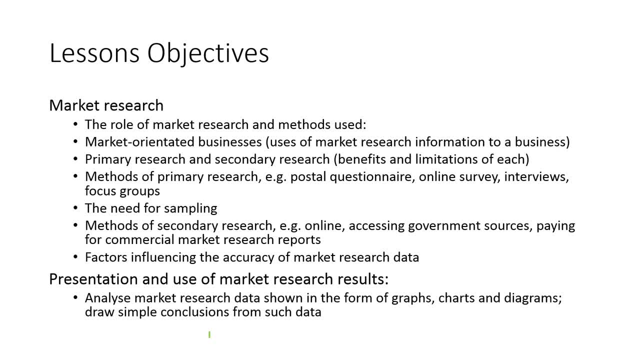 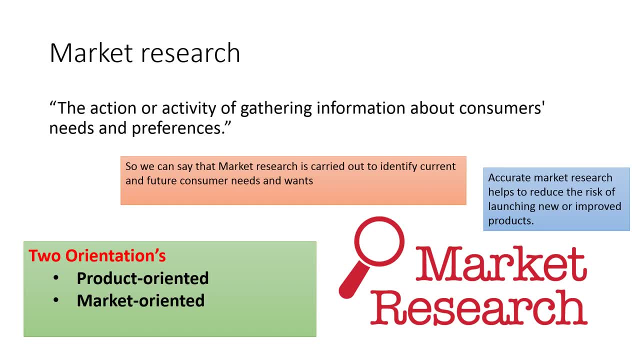 And then we'll move on to how is market data, or market research is presented and used by the market. So what is market research? It is the action or activity of gathering information about consumers' needs and preferences. So that is what a definition of marketing is. 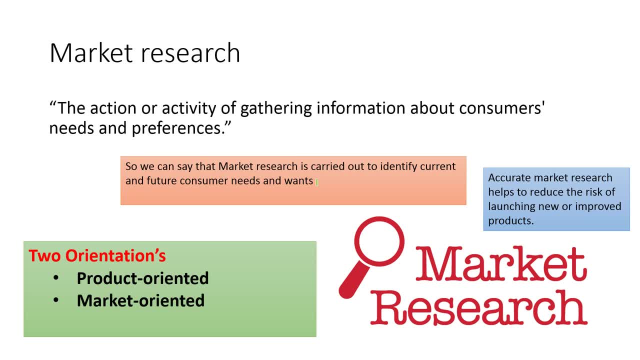 So we can say that market research is carried out to identify current and future consumer needs and wants. Does that make sense? Is that clear for you? So what marketing does is it wants to identify and Know everything, or as much as they can, about their customers. So accurate market research helps to reduce the risk of launching new or improved products. 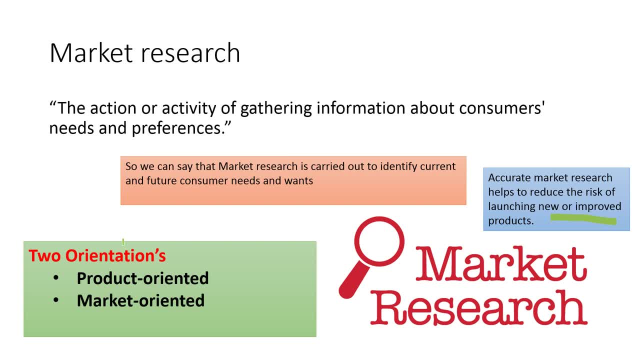 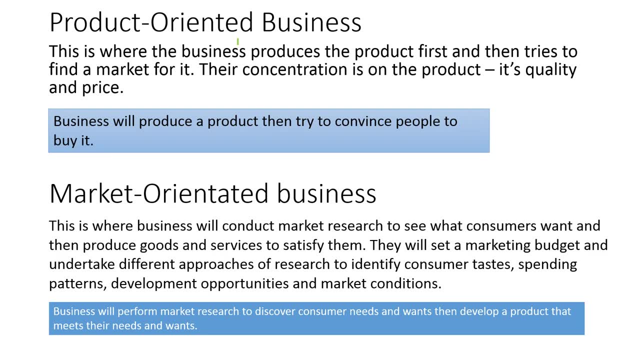 So there's two types of orientations we're going to talk about, That's, product orientated businesses and market orientated businesses. So product orientated business means this is where the business produces the product first. So remember: So it produces the product first and then tries to find a market for it. 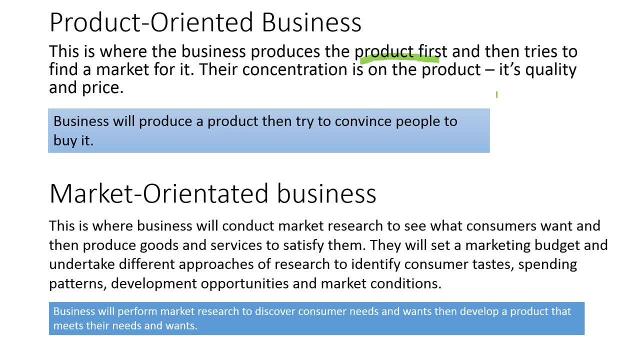 Their concentration is on the product, its quality and price. So business will produce a product, then try to convince people to buy it. That is what product orientated business do. And then we have market orientated businesses. These businesses try and will conduct market research to see what consumers want. 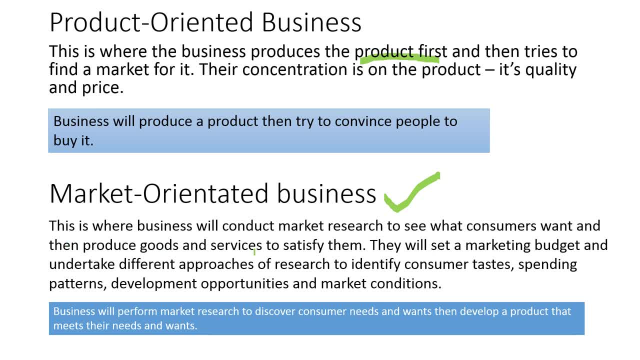 And, And then produce goods and services to satisfy them. They will set a marketing budget and undertake different approaches of research to identify consumer tastes, spending patterns, development opportunities and market condition. So in market orientated businesses business will perform research first to discover the consumer needs. 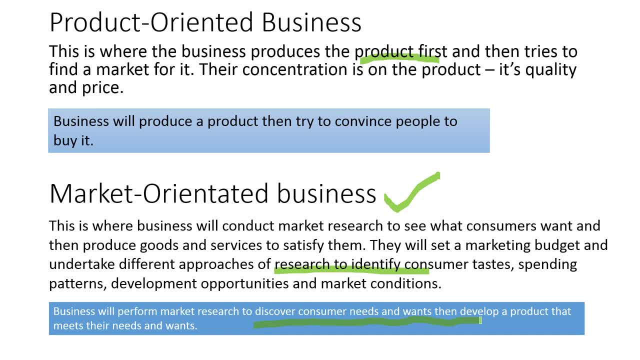 So market orientated businesses. Business will perform research first to discover the consumer needs, needs and wants and then develop a product that meets their needs. so here is a question: which type of these two businesses to orientation is better for a business? do you think it's better to produce a product and then just convince? 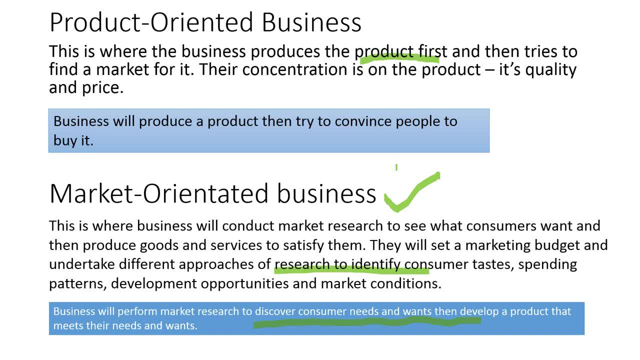 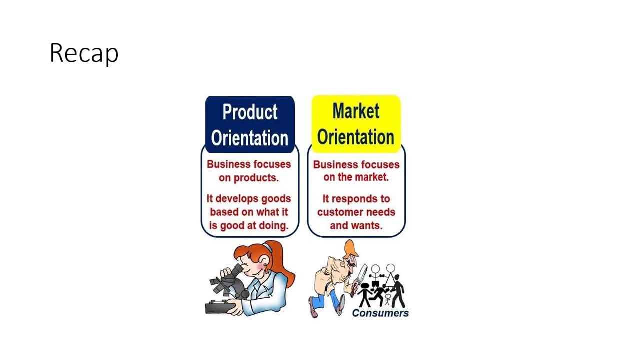 people to buy, or do you think a company should do some market research before buying a product? make sure your answer is at least 20 to 50 words and I will market in the comment section below. so just a recap now. so market product orientated businesses focus on the product. it develops goods based on what. 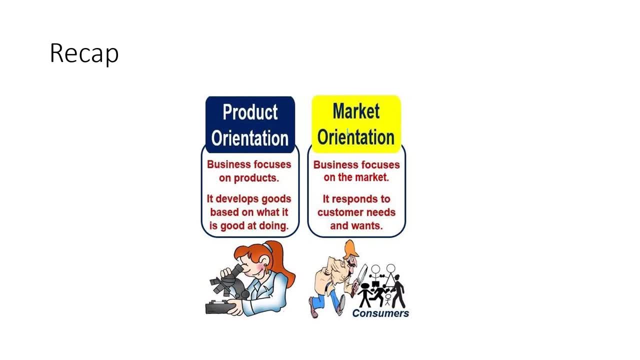 it is good at doing, and market orientated businesses focus on market. it depends, it responds- sorry- it responds to customer needs and wants. so that's what the difference between these two are. you need to remember that because they will, they might or will possibly come in your exams. so there's two types of 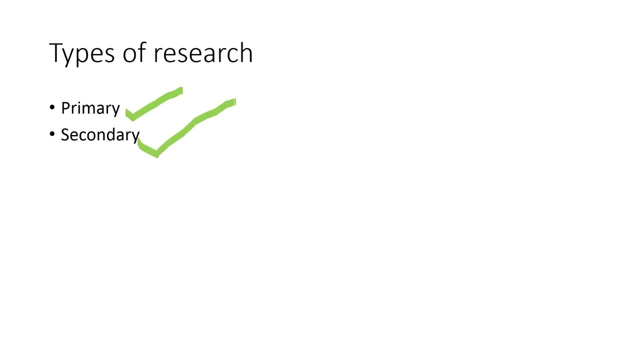 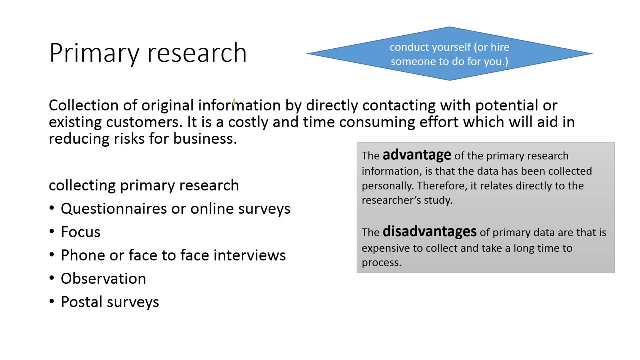 research. we're going to talk about primary and secondary. if you remember, we talked about primary, secondary, tertiary sectors in a earlier video. this is kind of same thing. so primary means original, secondary means the second, second original, if that makes sense. so what is primary research? collection of original. 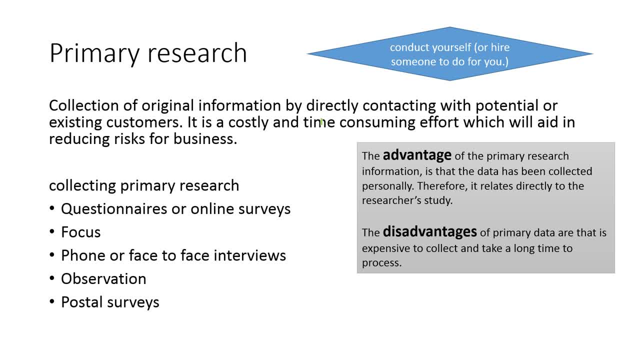 information is based on the research that you have done in your previous years. so what is primary research? collection of original information is based on the by directly contacting with potential or existing customers, so it's the collection of original data. it is costly and time-consuming effort, which will aid. 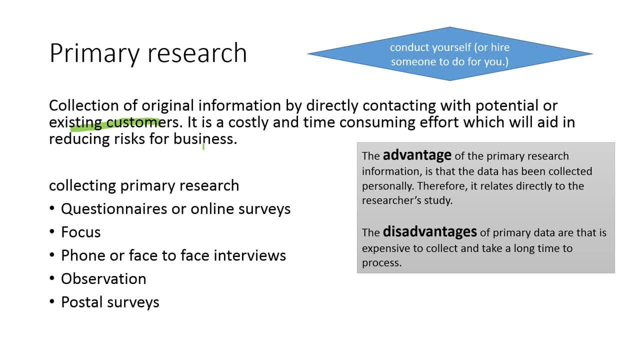 in reducing risks of for a business, so it can be very costly and time-consuming. so that is some of the downsides of primary research. so primary research is conducted by yourself, or your hire someone to do it for you. the advantages of primary research is that the data has been collected personally. therefore, it is really it relates. 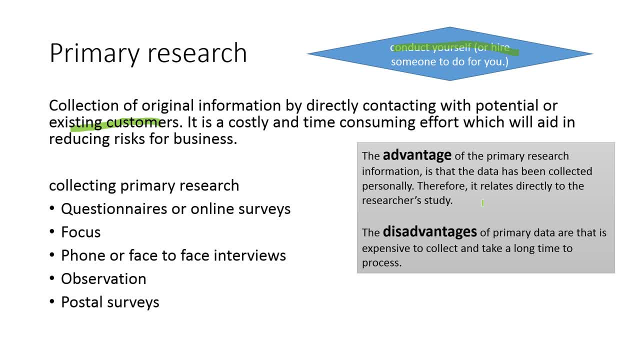 directly to the researchers study. so if you do or collect primary research on a project, you're obviously going to relate it to a topic that matters to you and the data is going to be related to that topic. so how there's a disadvantage. I've put here for years old just in case, so you know. 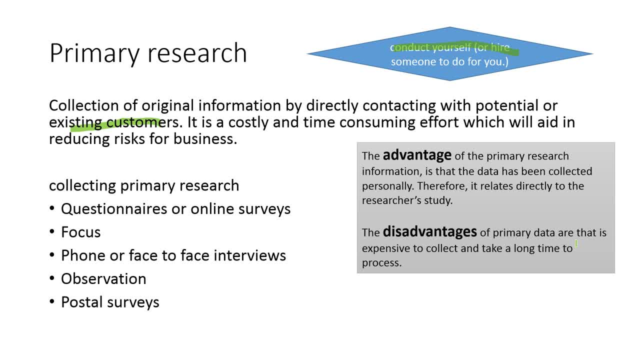 about it. the disadvantage of the primary data is that it is expensive to collect, collect and it takes a huge amount of time to process because you need to put them in order, and so on. there's a lot of effort that goes into primary research because, after all, there's nobody else that has collected such data and you are. 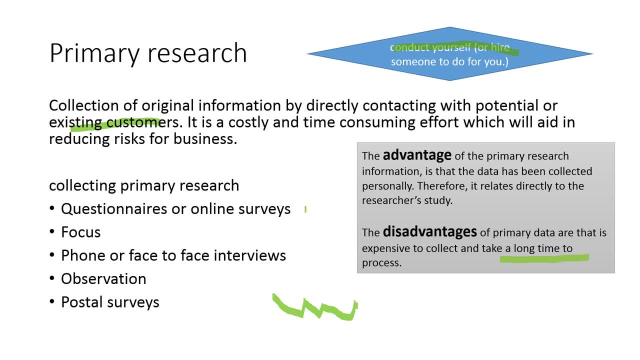 the first to to do it, so it will require a lot of time. So how could we collect primary research? So we could do it by questionnaires in an online service. We could do focus groups to collect the primary research. We could do face or over the phone interviews with our customers or with potential customers. 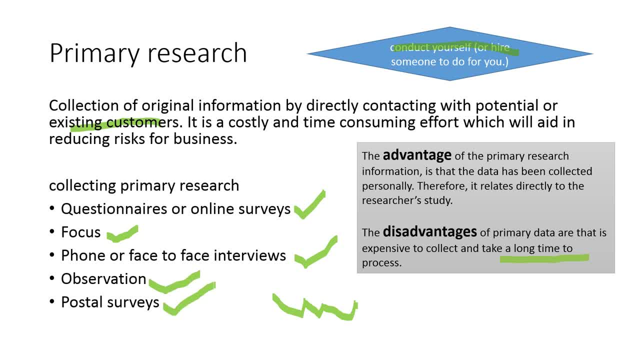 We could do observation, We could do postal service. So there's a number of ways we could obtain primary research. But what you need to remember is that not everybody will be honest when they are doing review. So, no matter how good you try, your data is very likely to be about 20% accurate. 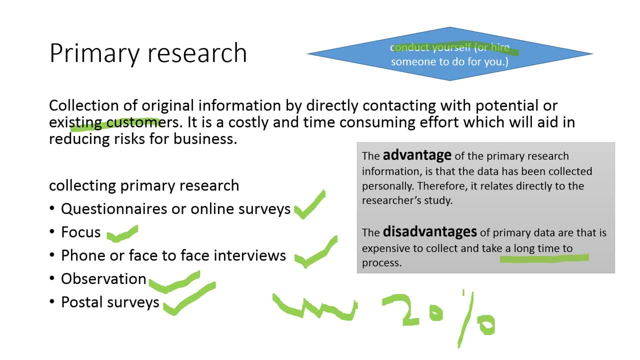 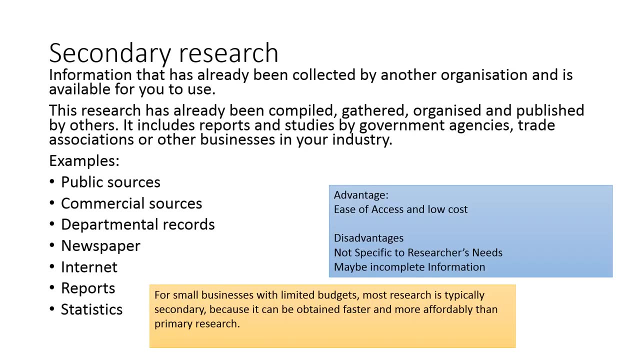 So that's not a great amount of percentages there. But according to some online studies that I've done in some books, no matter how good you try, your data is going to be no more accurate than about 20%. So secondary research is information that has already been collected by another organization and this is available for you to use. 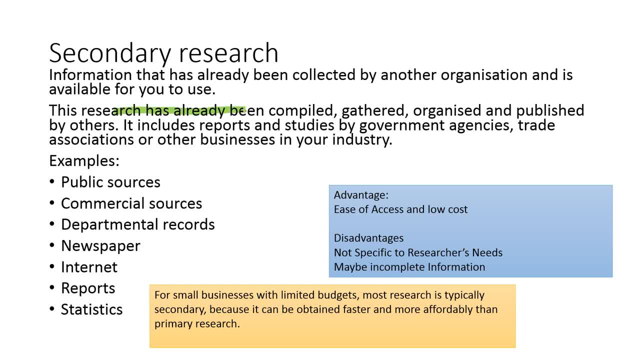 So this research has already been compiled, gathered, organized and published by others. So secondary is already been organized and it's published and it's just ready for anybody to use. for small businesses particularly, It includes reports and studies, Studies by the government agencies, trade associations or other businesses in your industry. 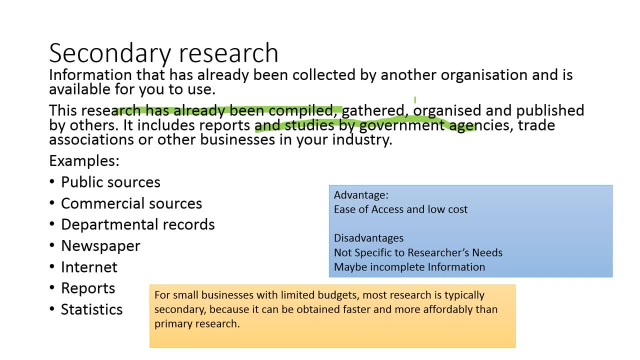 So secondary research is. so you might be working in a cake factory, for example, So there will be some other companies that have already collected such data about what sort of cakes people like the most. So that would be a secondary, Or you could do your primary research and ask your customers or potential customers by giving them some. 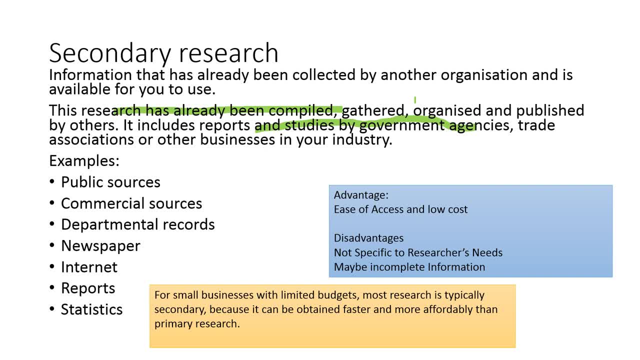 Questionnaires or interviewing them or sending them postal service. So you could either use primary research collect yourself, or you could get some secondary research from other resources or companies. So the advantages of secondary research is that it ease of access and low cost. 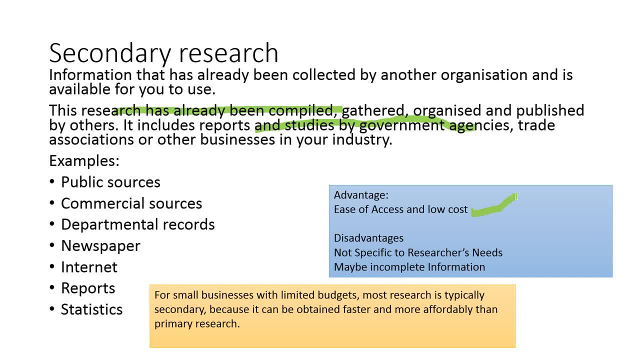 So there's some doesn't even cost you anything, Whereas primary would cost you a lot of money. This doesn't really cost you that much money. Some, most especially government agencies. they provide lots of reports for free. It's on the website. 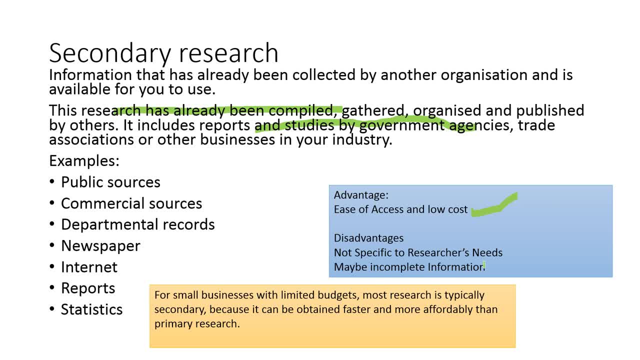 The disadvantage is that not specific to researchers need, So maybe incomplete information. So the research that has been gathered it's for another agency, It's for an overall observation, So it will not be related to your company. For small businesses with limited budget. 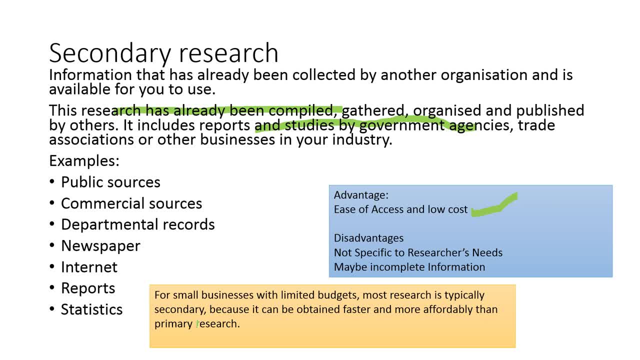 Most research is typically secondary because it can be obtained faster and more affordable than primary research, Just like I said earlier. So it is very easy to get secondary research than it is to get primary research. So how could we get secondary research? We could public resources sources. 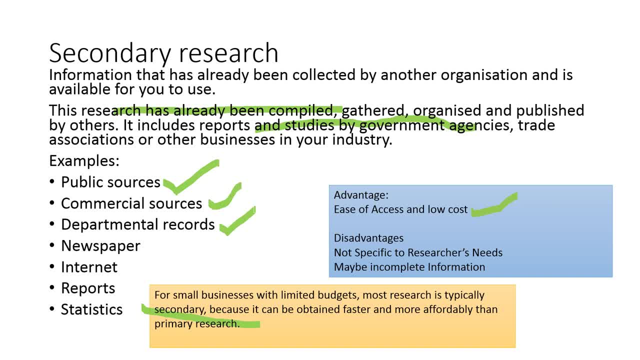 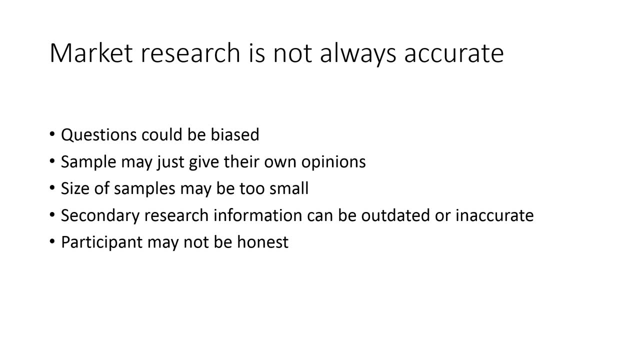 We could have commercial sources, departmental records, newspaper, internet. We could report statistics. So government statistics, government reports, We could. there's a number of places we could obtain secondary resources. So depends on what you would, What sort of data you're looking for. 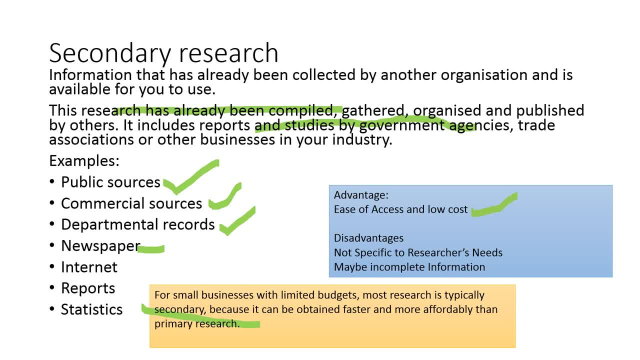 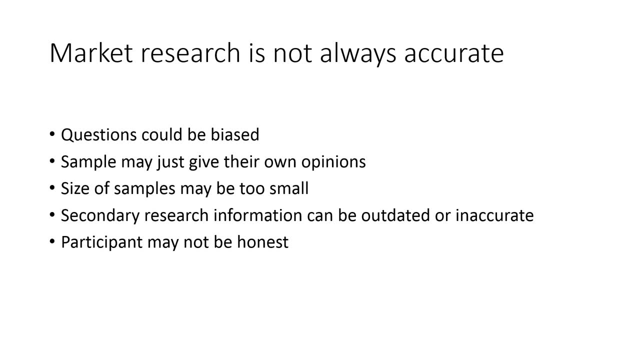 You could go on to different websites or different organization who have already done it, and you will be able to obtain such details. A library will be a perfect place to obtain lots of research or documented research About certain projects. so what market? so market research is not always accurate. 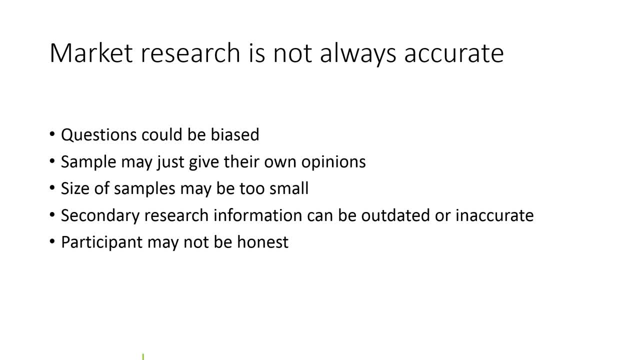 or, like I said earlier, according to money online websites, that only 20% of it is accurate. so so the questions could be biased. so the question that we asked the customers could be or potential customers could be biased, and that is why we will not get an accurate market research. so sample may just give their 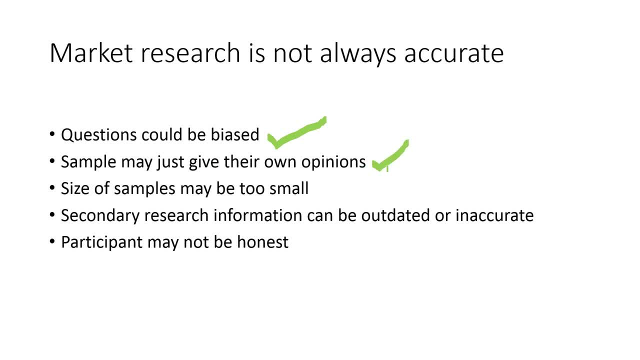 own opinion. so if we sample some people they will just give their own opinions. you know, not represent the whole group, so size of sample may be too small. so if we're gonna sample five people to represent a hundred thousand people, the sample would be too small to accurately represent them. so secondary research. 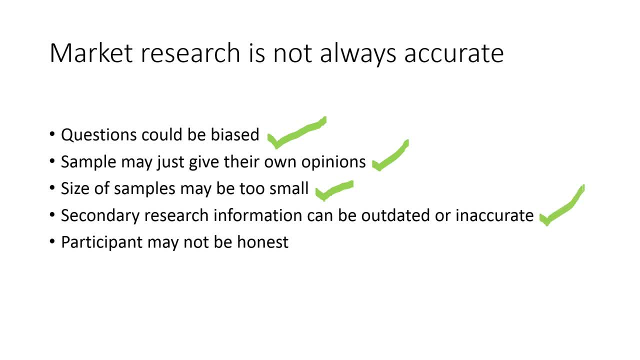 information can be outdated and incorrect. so some research will take two, three, four years. so by the time you get your hands on that research it will be outdated and probably inaccurate. so participant may not be honest, so they might not answer question honestly. they'll just put yes, yes, no, no, no to everything, to just 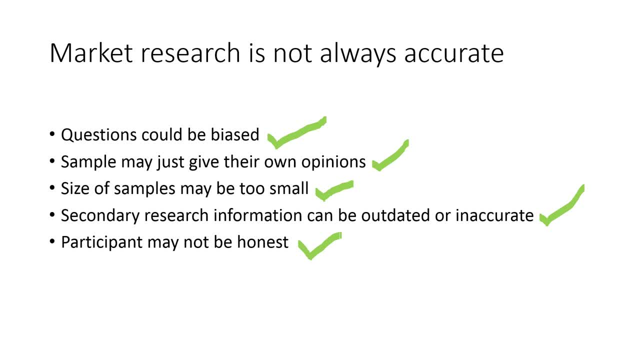 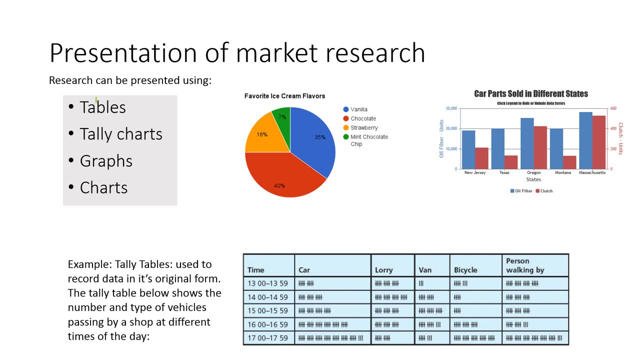 quickly get the question or the survey completed, you so that is why the information is not always accurate. the market research information- so how can we present market research to X- is presented by tables, tells, classified. we can use chart, so there's a number of ways we can present. 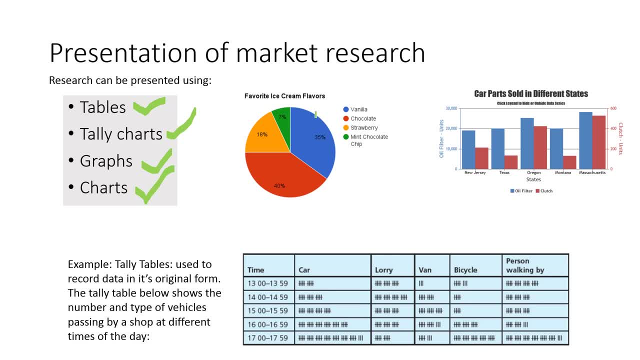 market research. so here, for example, to find out. so we have some information about favorite ice cream flavors. so we have got vanilla chocolate with入 уш i strawberry mint chip, mint chocolate chip, so we can present that in a pie. then I've got some car parts sold in different states so we could identify. 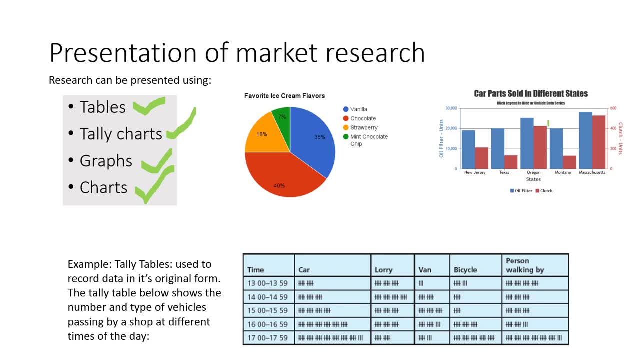 what cars were sold and where, and we could use a graph to present such information here we could. we have used a tele chart to represent some more information to record original forms. so the tally table below shows or shows how many different types of vehicle past the shop at different times. so do you see? 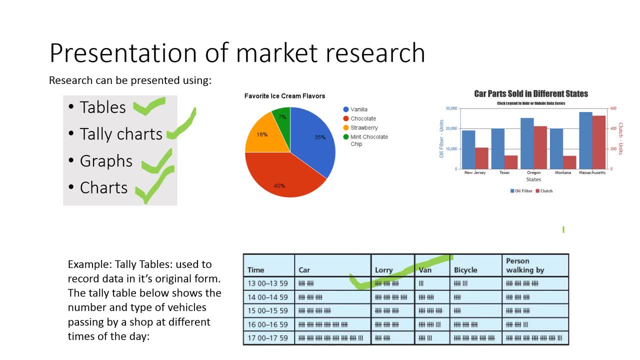 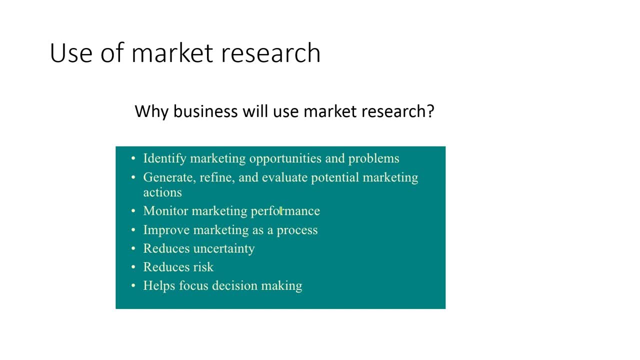 there's a number of way we could present market research. so use of market research why businesses will use market research. they use it to identify marketing opportunities and problems, to generate, refine and evaluate potential marketing actions, monitor performance, improve marketing processes, reduce uncertainty, reduce risk, help focus decision-making. so there's unlimited ways that businesses will use. 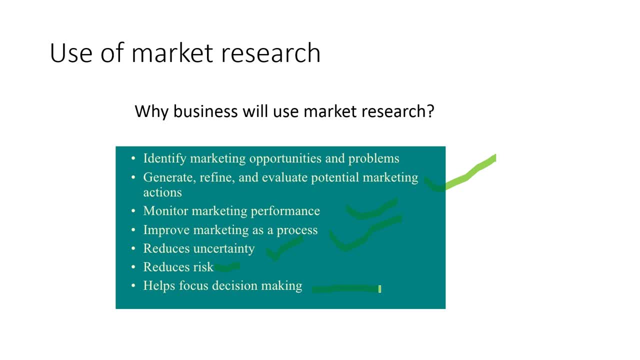 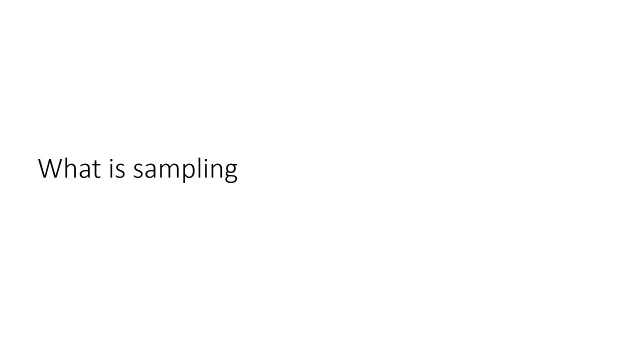 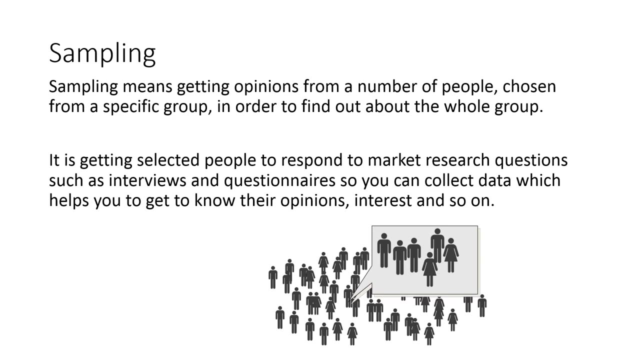 market research to help them make decision, create products that help the customers and meets the customer needs. so what is something? not so now that bring us to something. so what is something? something means getting opinions from a number of people chosen from a specific group in order to find out about the whole group. it is. 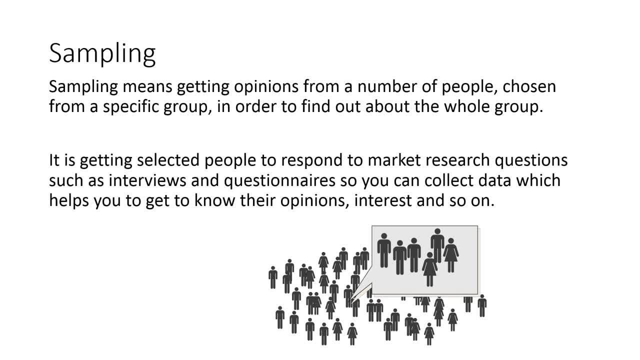 getting selected people to respond to market research questions, such as interviews and questioners, so you can collect data which helps you to get to know their opinions and trust and so on. so sampling is: this is the whole group and we can get five or six people to represent this whole population for. 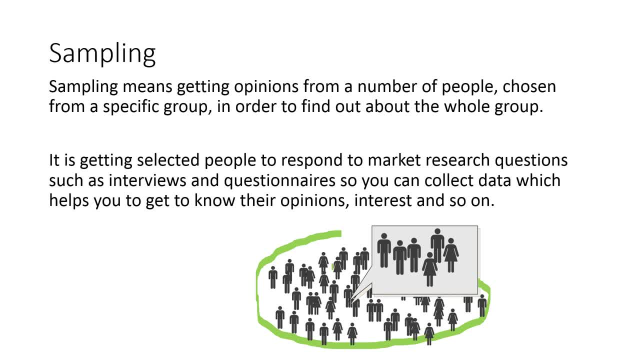 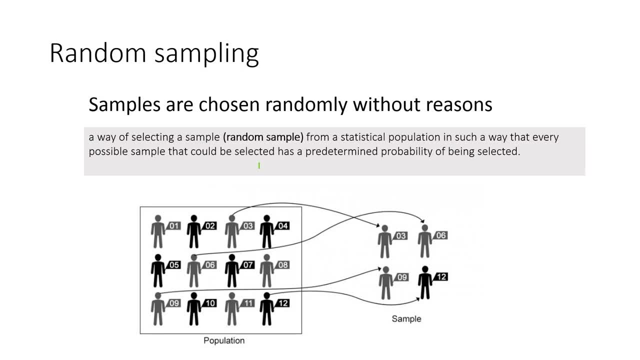 example. so sampling is basically just getting random or selected people to represent the whole bunch, whole group. so there's a random sampling. so samples are chosen randomly, without a reason, without reason. so we have a sample, random sample from a statistical population in such a way that every possible sample that could be selected has a predetermined probability. 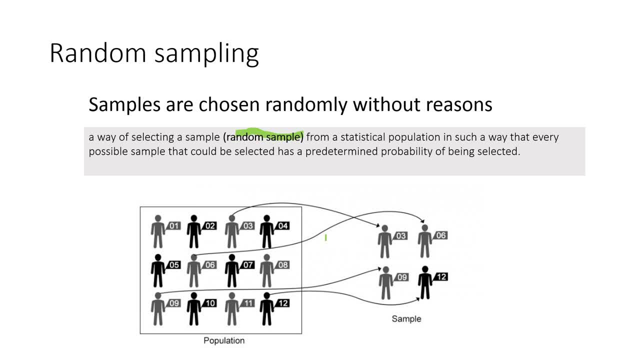 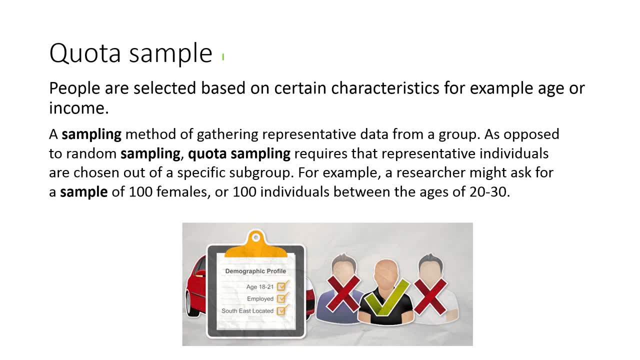 of being selected. so we could use such way to do random sampling, or we can do quarter sample. so this is where people are selected based on certain characteristics, for example age or income- a sampling method of gathering representative data from a group, as opposite to random sampling, quarter. 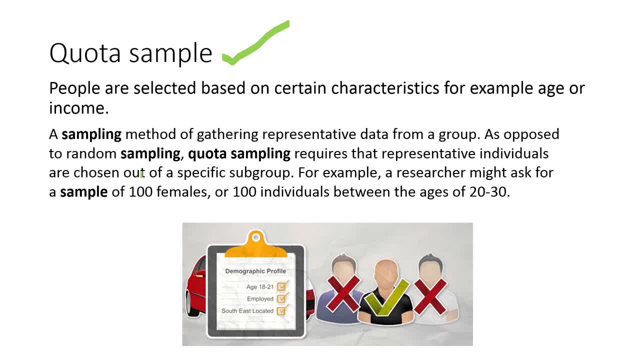 sampling requires that representative individuals are chosen out of a specific subgroup. so do you remember? whereas in random sampling we're just picking people, here we need to get individual that are selected from a specific subgroup. for example, a researcher might ask for a sample of 100 females or 100 individuals. 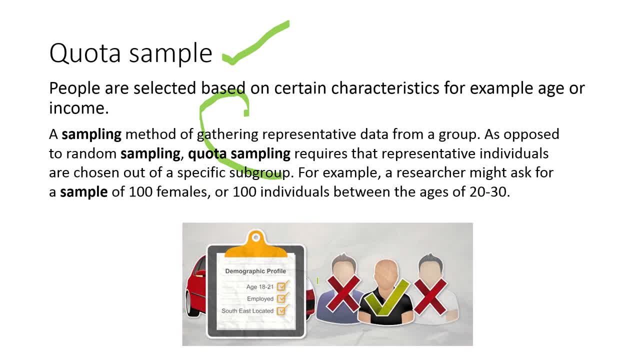 between the age of 20 to 30, so I've put a picture here. so what? we have got three people here, but what we are looking for is someone that's aged between 18 to 21, is employed and is located in southeast. so this gentleman is matching our. 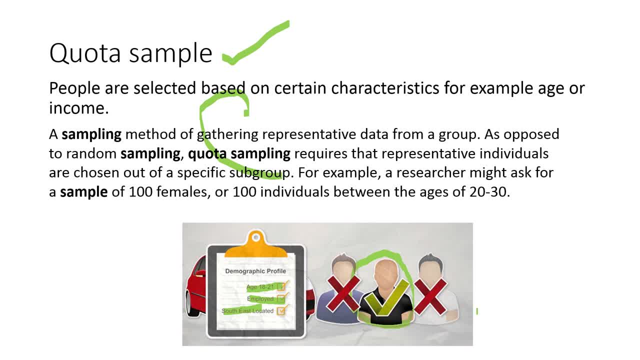 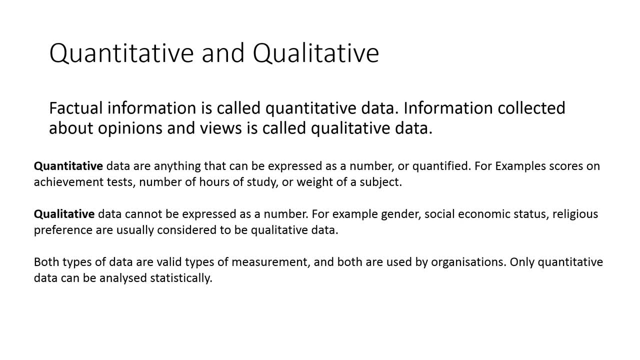 criterias, and this is what's called quarter sampling, and we would ask him to contact this person, raise your hand, so, and there you have the information upon which you can note down the number of events that occurred in this subgroup. so now I'm settling in with the lambda stamp because our transcript danette. 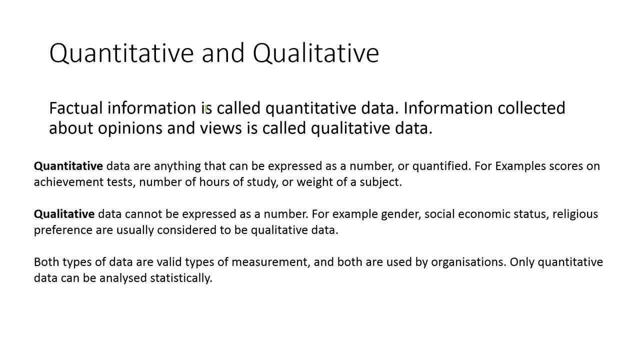 doesn't care, so we'll go back to our answer book. so now let's check whether this is the number that strangers have served我们的顾问هم, and there it is. so if he's a tubes from The perfect's use is called quality, so quality data are anything that can be expressed as a number or 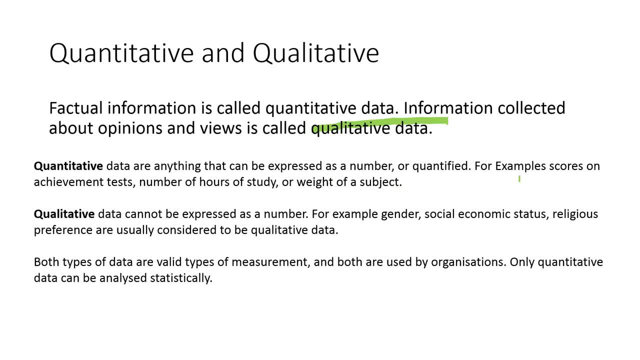 or quantified- for example, scores on achievement test, number of hours of studies or weight of a subject- whereas qualitative data cannot be expressed as a number, for example, gender, social, economic status, religious preferences, or usually considered to be. these are all usually considered to be qualitative data. so both types of data are valid types of measurement and both are used by